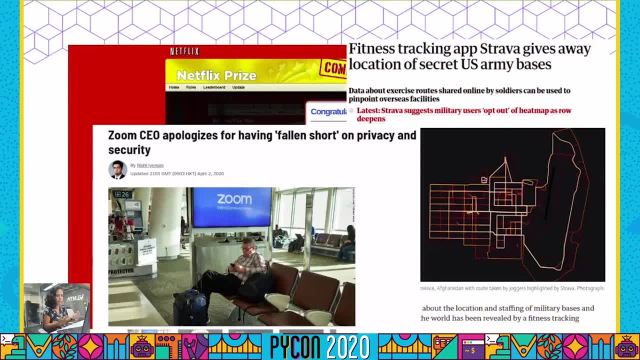 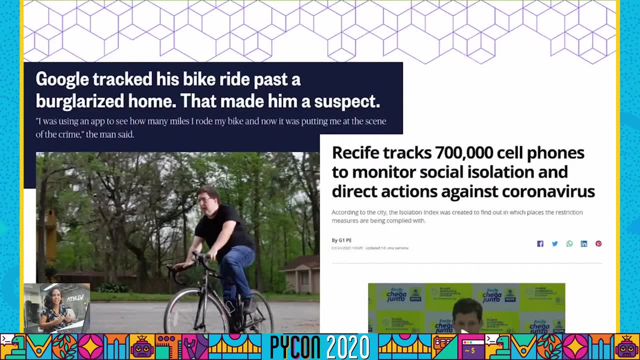 more privacy while using like applications and systems, But I don't know what you think about that, but I don't know if any good came out of this We have. I bring to you two examples of a guy who just used an app to track like his rides on his bike and that made him like: 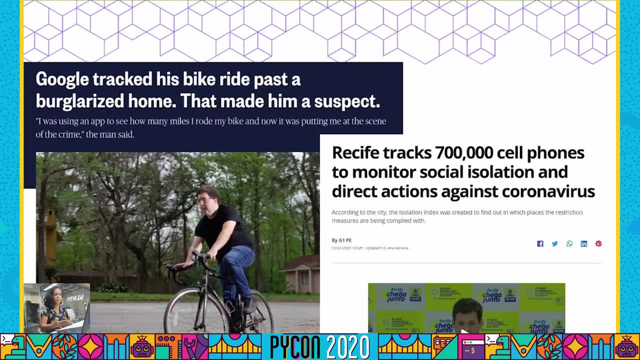 a suspect of a robbery, And this is an example from my hometown where they are using like mobile phones to monitor social isolation. I don't know how you feel about that. You may feel that the government has the right to do this to citizens, but it's a debate that 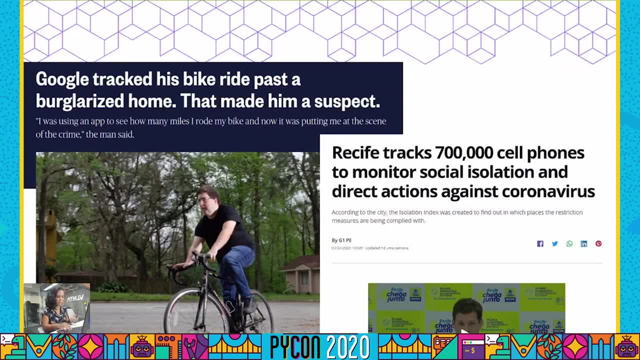 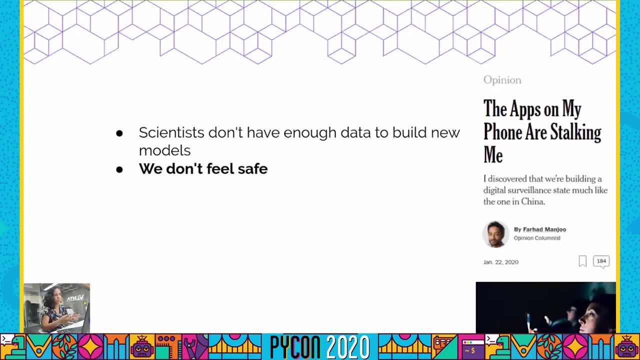 we need to have as a society And the consequences of all these like debates and discussions is that first scientists: they don't have enough data to build like new models. And then they build new models because, basically, all the most important data is in the hands of big. 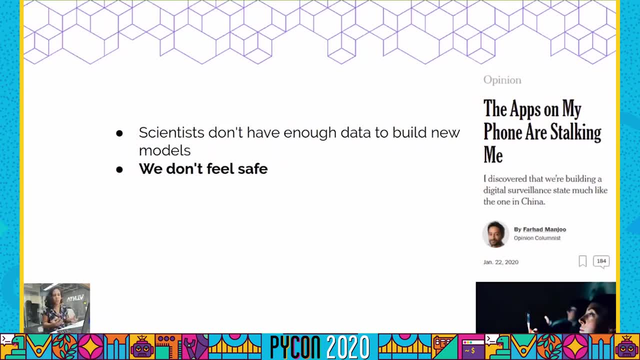 companies, And I think the worst thing is that we don't feel safe. We think that we are being watched all the time and it's like we can't do anything to solve this And all I can just talk to show you that there's a few things that we can do and I'll show you. 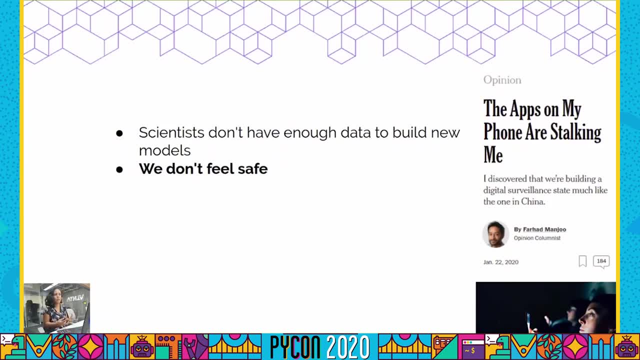 a few situations when we can hurt the privacy of users, but I'm going to show you ways on how you can protect yourself And I'm going to show you some simple examples and then we're going to go to more like complex situations. So I would like to start with a very simple situation, like you want to collect. 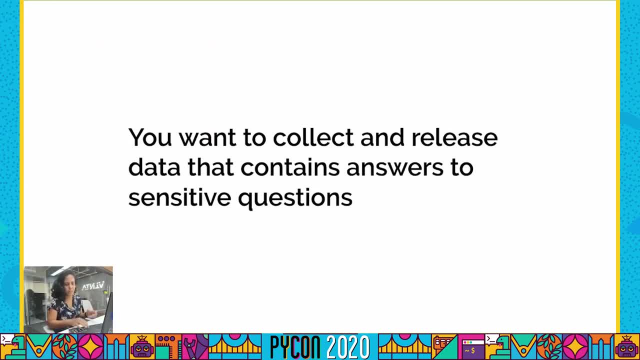 and release data that contains answers to sensitive questions. So you have, like, a group of people who have a lot of questions that you want to ask them and you want to put these results on a database and then, just like, get statistics out of it. And then you want to. 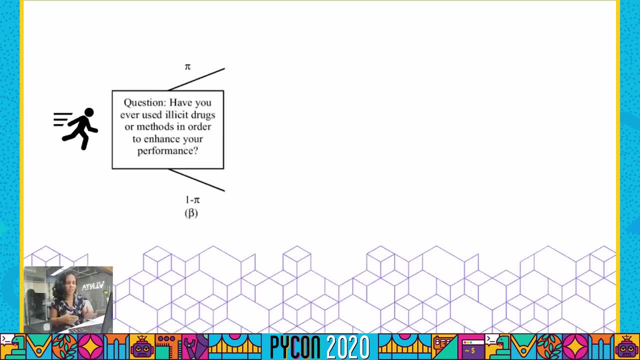 ask them what they think about this. When I say sensitive questions, I really mean sensitive questions Like: assume that I'm an athlete and I'm going to ask like questions like: have you ever used illicit drugs to enhance performance? We have two options. We have like a clean athlete. 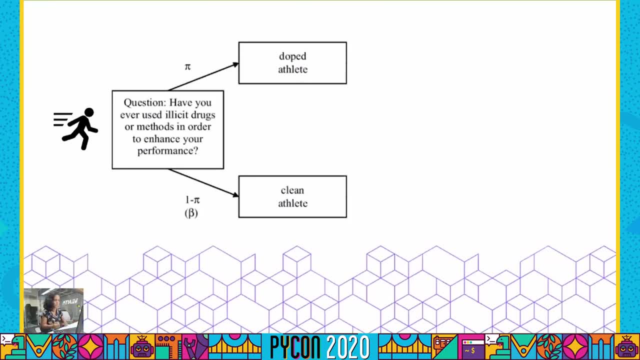 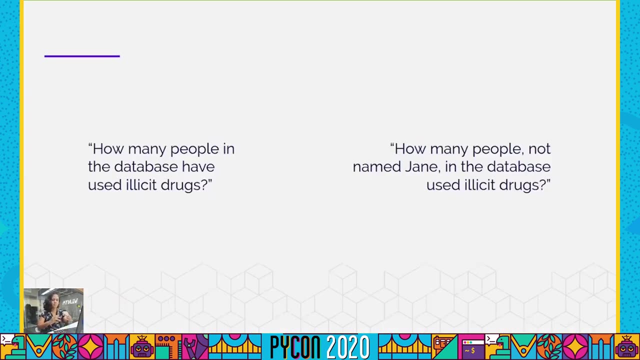 that didn't use drugs and we have an athlete that may have used drugs or used drugs And, assuming that these people answered the question honestly, we will have like a database and we will be able to do like queries on this data set. But there is a problem with that. 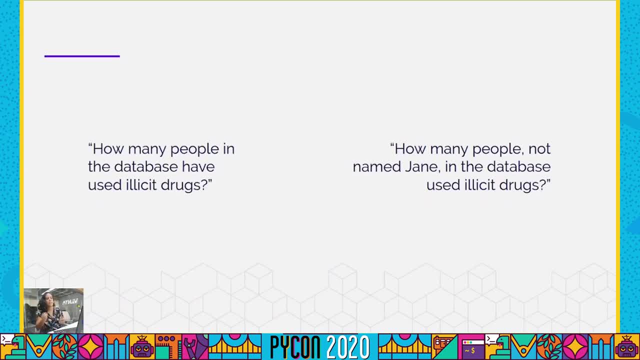 and it's kind of: if I allow people to just get statistics from my data set, it doesn't mean that I'm protecting privacy. Just by not allowing them to get individual's names doesn't mean that I have privacy. In this example, you can see that with two questions. 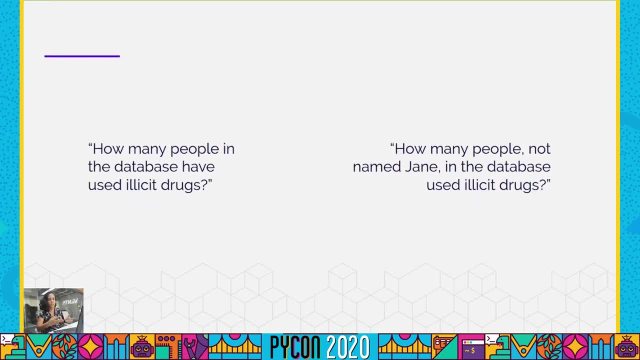 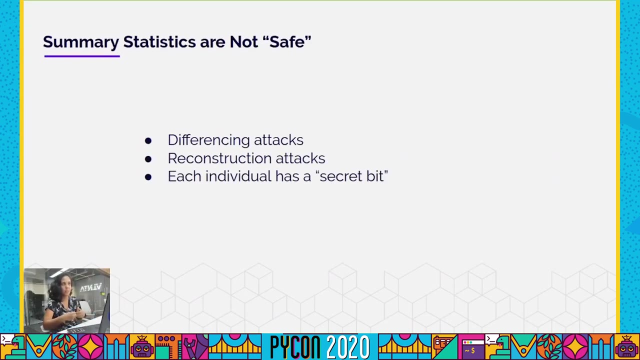 I can know for sure what it is if Jane used or did not use illicit drugs, And that's it. That's why statistics are not safe. The name of this attack that we just simulated by asking different questions is called a differential attacks, And we can do many more types of. 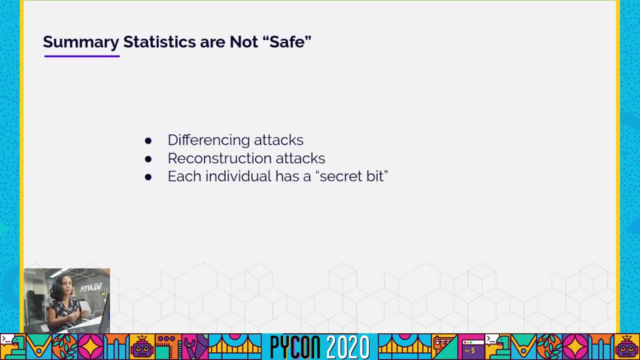 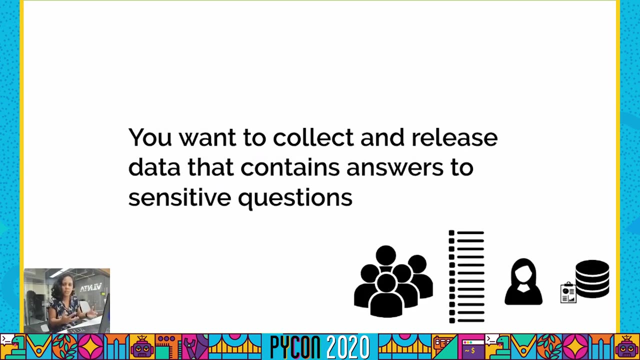 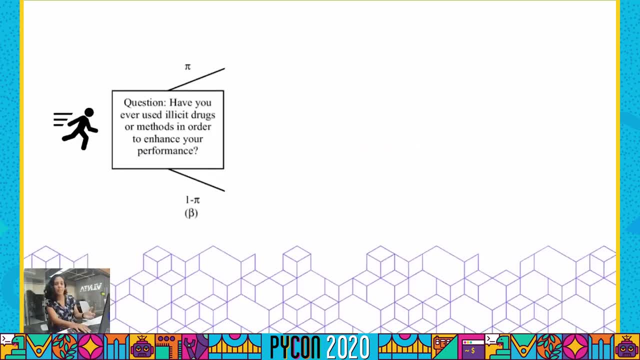 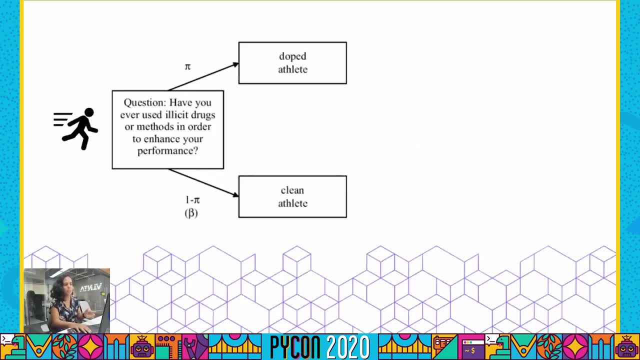 the same question and we still have two options. The difference is that now I'm going to just something at data collection time, So I'll give the user, the athlete, a coin and I'll say: Flip the coin. Now let me see the result If the coin is head. so you will answer Yes. 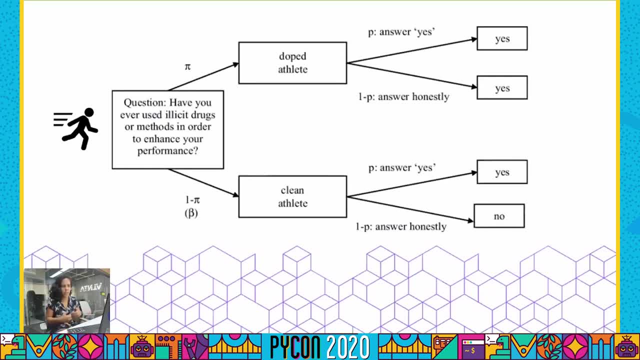 coin is still going to say: answer honestly. and this would make the clean athlete and the dope athlete both answer, I guess under certain conditions. so we are giving, like the, the people in the research, a type of plausible deniability of the presence of, if they use or 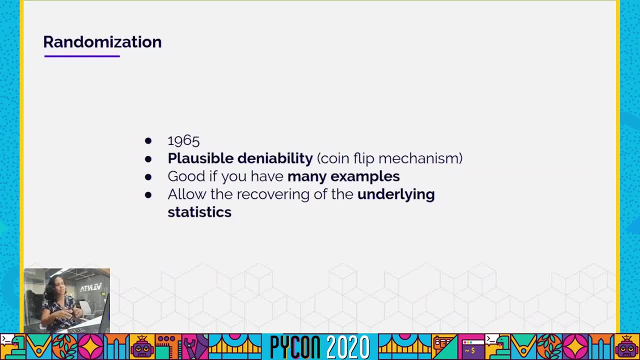 do not use this interest. the idea of this technique is called randomization, is a technique used a lot in the 60s and the idea is that people could not answer questions honestly without being like held accountable, without being like suffer some kind of prejudice at that time. so they 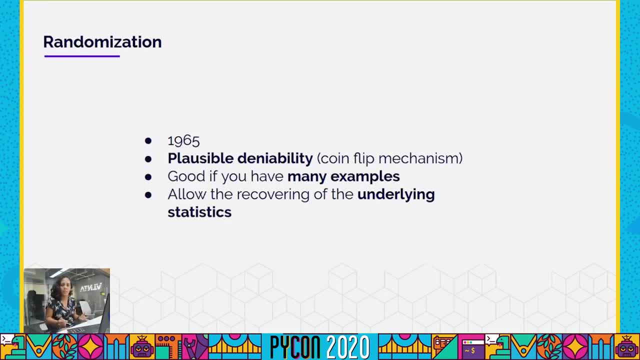 developed this mechanism to give people the possible deniability by. you know the coin flip and it works very good for have many examples and it still allows you to curve the underlying statistics so you can get the mean. you can get the percentage of users. they use, one, what we did not use and every other. 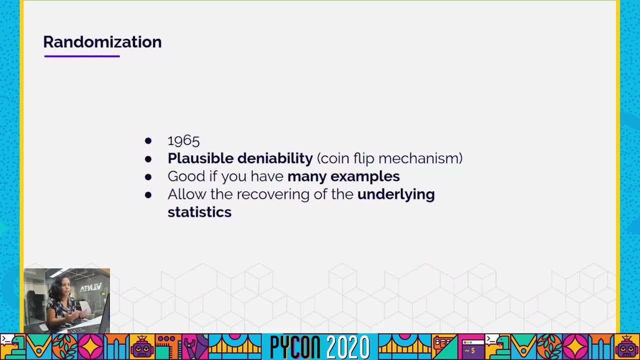 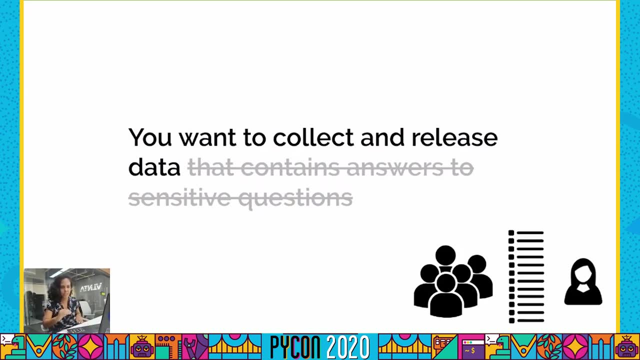 information, statistical information that you would like to like collect. but let's put this type of sensitive questions aside. you don't care too much about that. you want to just collect and release data because it's important for you, because you have a partner. you have to share this information with your partner, or you have like a 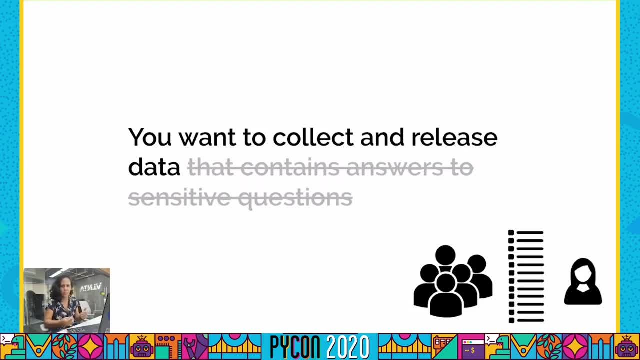 third party that provides you a service and you want to just get the result, or you want to share for some research example, like the applications are, uh, mainly, and what could happen is the first thing that you will do will be like remove names and remove social security numbers. but there's a 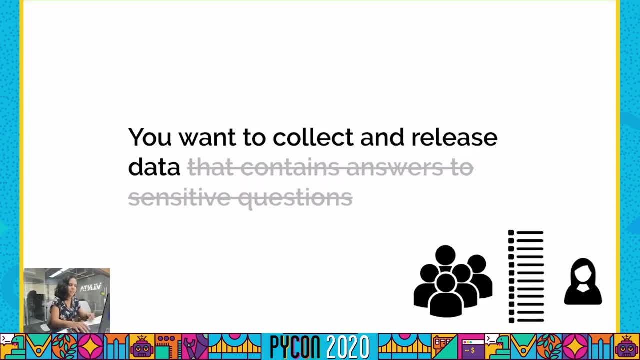 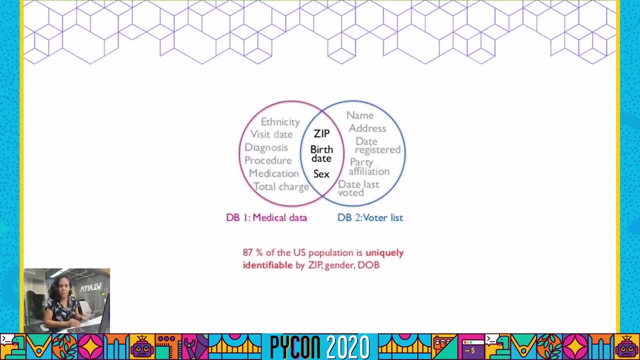 few things that you need to think other than this: few attributes that they are calling quasi-identifiers, and they are, by itself, not unique. many people may have them, but the idea is that when you put these attributes together, they can give enough information to identify a person Here, for 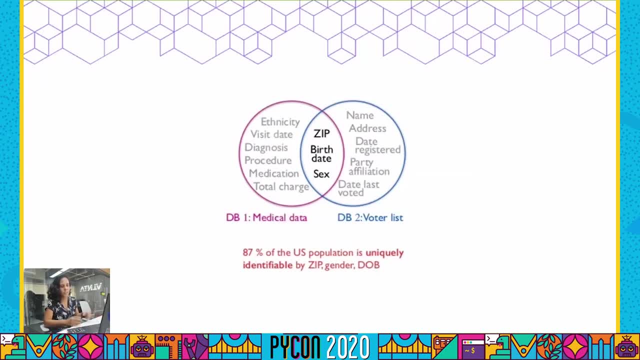 example we have 87% of the US population can be uniquely identifiable by zip code, by gender and date of birth. So with this information we can get all. we can identify one person in a database and this gets a bit more tricky when we join. 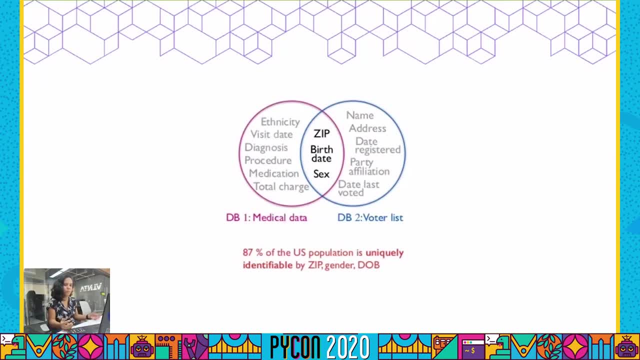 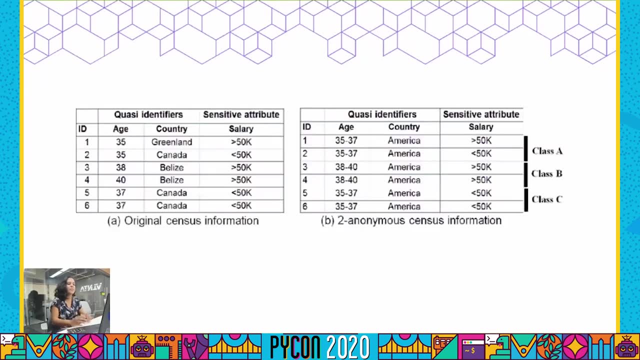 database So we can get, with this information, we can get all the information of a person's life, which is, I think, a little bit critical. you know, One way to solve this is here we have quasi-identifiers as age and country, and 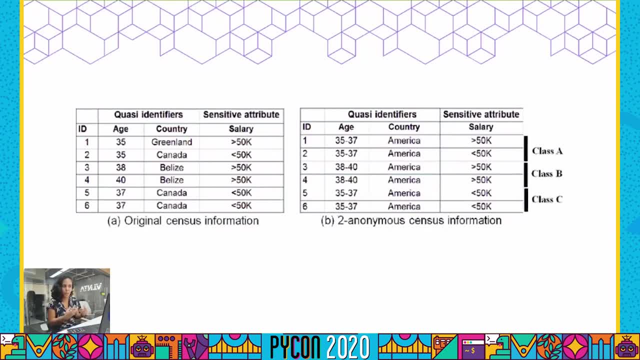 we have a sensitive attribute. they want to hide this attribute. we don't want to let people know the salary of those other people, and what we will do is we will like pair the quasi-identifiers and the country into general groups, So we will make people. 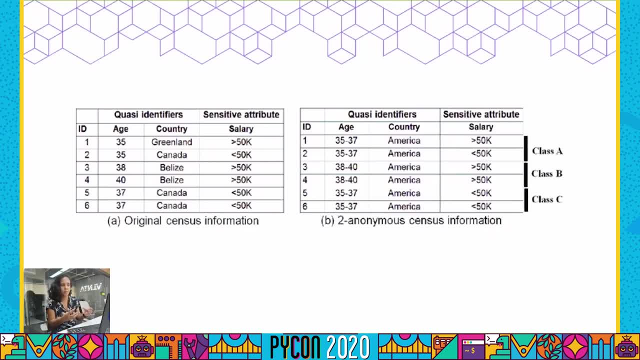 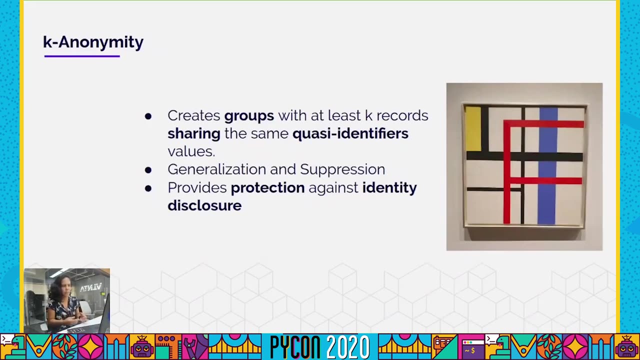 fit in groups and we have people- more than one people- in one group, so we cannot point to the people directly in a database, And the technique that does that is called key anonymity. the idea is that you can create groups with at least k people that share the same quasi identifiers. 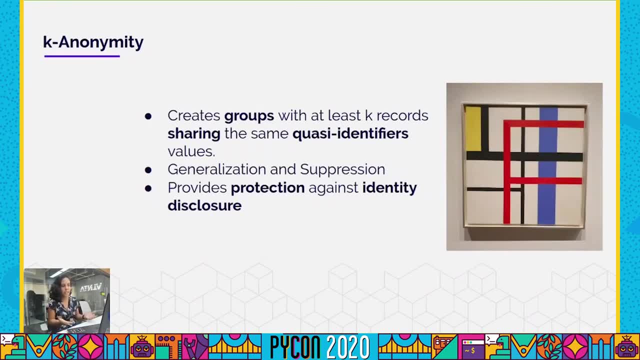 so you cannot just point one person by looking at the table, and we can do this by using generalization, that is, we will just get an attribute and we will like change the granularity of the information. or we can do this by suppressing information, by removing information that we think. 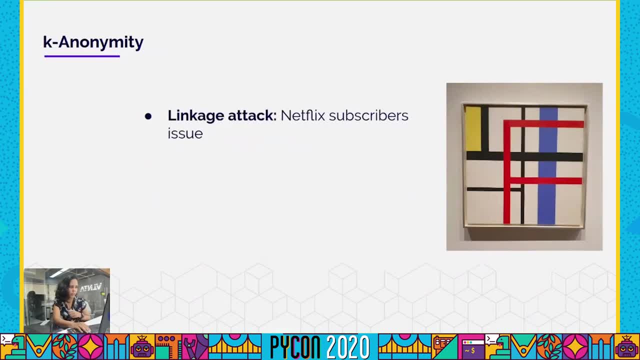 that links too much information. uh, there's still a problem that is linkage attacks that we can like. uh, some other future data may appear and then boom, uh, you have a private speech. there was like an issue like this with the netflix subscribers. you can see, it was like a context that they made. uh, 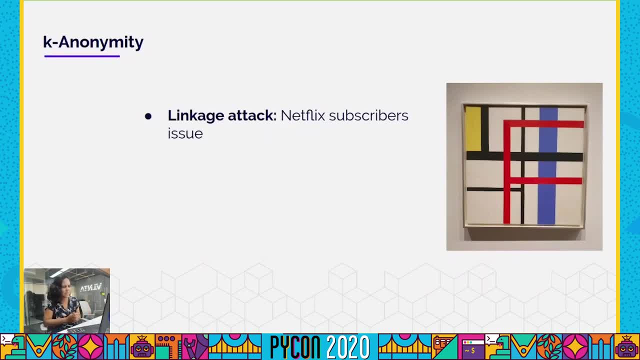 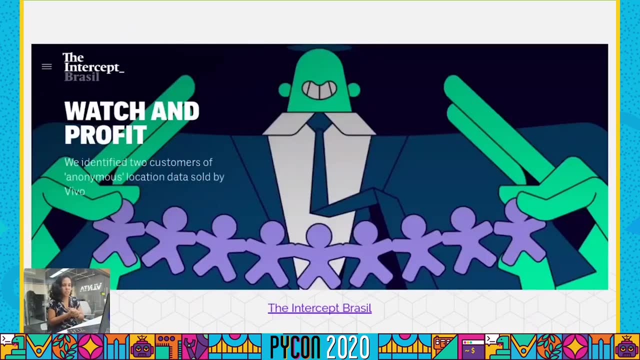 i think in a while. i don't remember exactly the date, but i have a very similar example that is quite recent, you know. i want to talk about it just a little bit. uh, in brazil we have a big company called vivo and they just released a data set that was uh anonymized, and they sell this data. 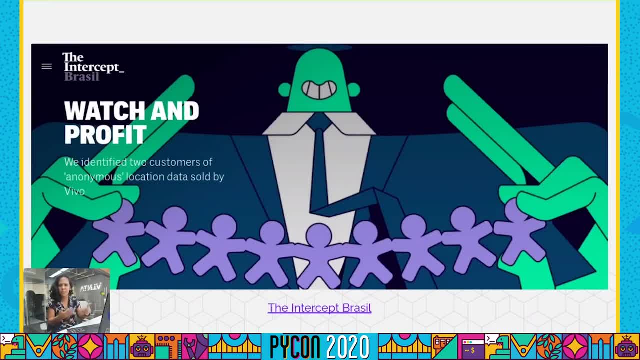 site to like the government and everything, and this data set became public and then some journalists were able to identify like two or three persons in the data set by linking the data that was public with data of concerts or something like that. there's a link and here and you can see exactly how they did it, but the idea is that, even though 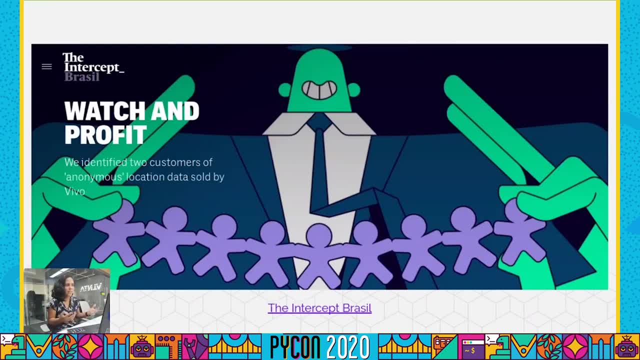 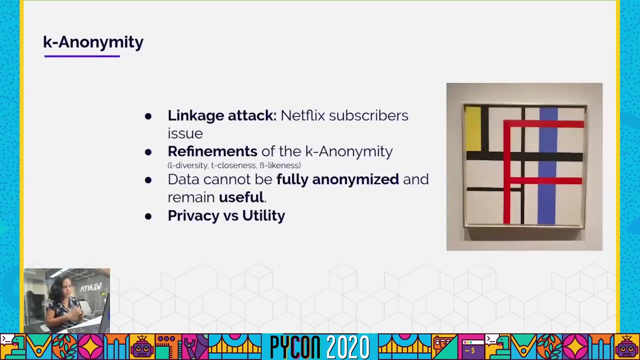 you think that you anonymize your data. you can just like be. uh, at some point, some other data may appear and people may be able to draw connections between the data. that's why, uh, you have to be extremely careful when releasing data. uh, there's a few refinements of canon in order to like protect against these types of attack. 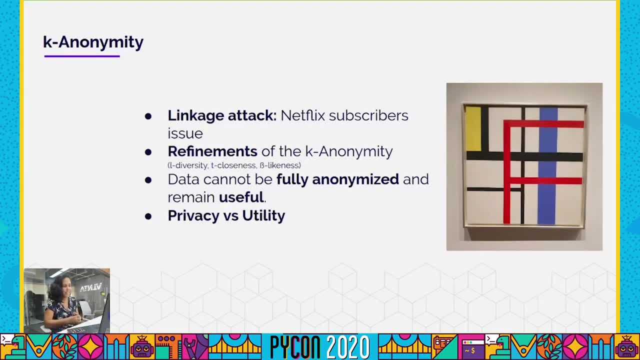 but they are all not perfect, and i would like to just point that you always have this trade-off between privacy versus uh utilities, so usability uh against privacy. you cannot minimize data and remain useful, so this will always be like a risk uh standing on your shoulder when you are releasing data sets in this manner. uh. i also have a few more examples. 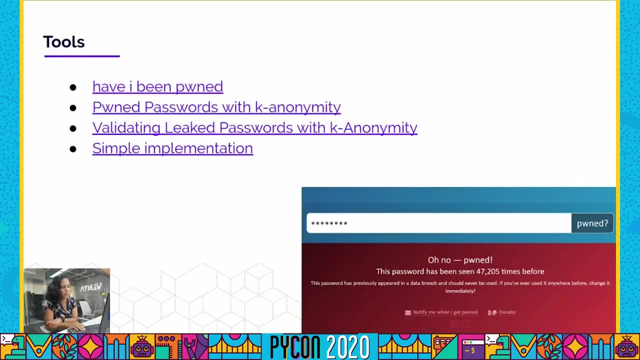 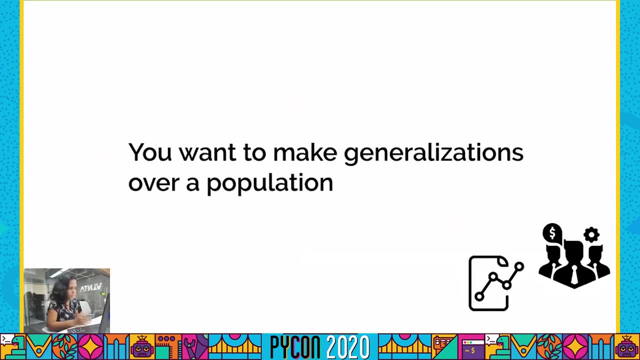 of applications they use. can i mean one? one example is they have have a big problem solution. i will leave the links here so you can check how it happens and how is the implementation, and i also have a secret limitation. you can check that later. another situation that i like to talk is you don't care much about releasing data you have. 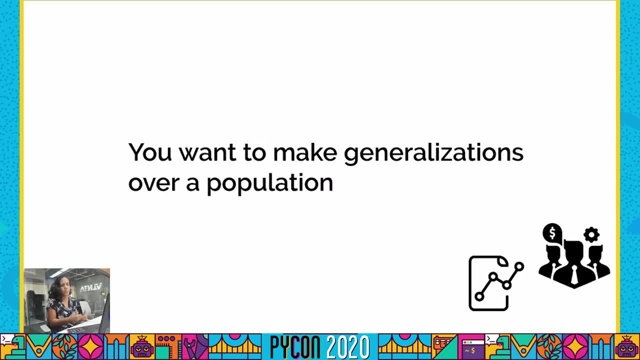 a data set, but i want to make generalizations over a population. how could you do that? sometimes you're not able to get more data and you want to know how to do that. the other thing is the data step sometimes is important. you want to know if you should launch product a, product b or you want to 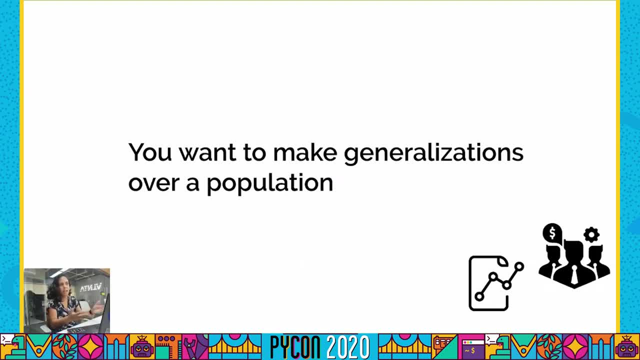 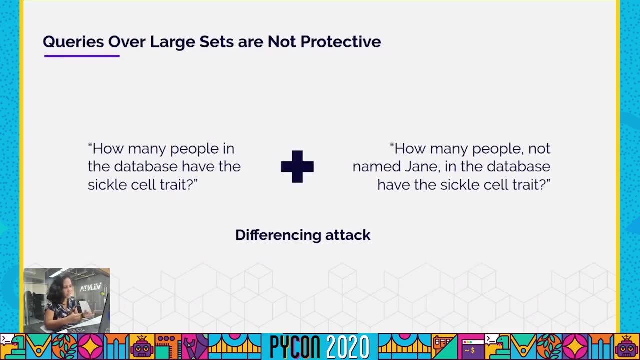 know, like uh, which, where your clients are liking the most. you want to make like general consults over your data set. how should you do that? in a private manner, because you remember that we discussed that we cannot allow people to do many statistics, statistics on the data, because we can. 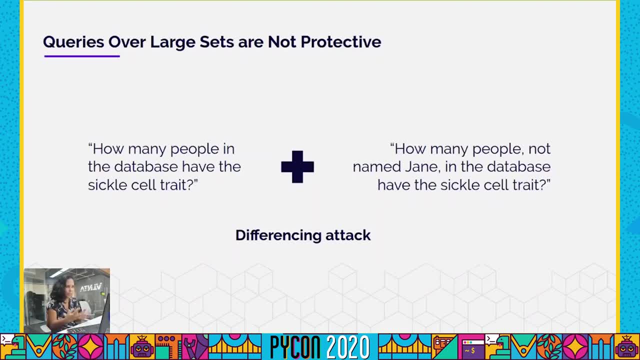 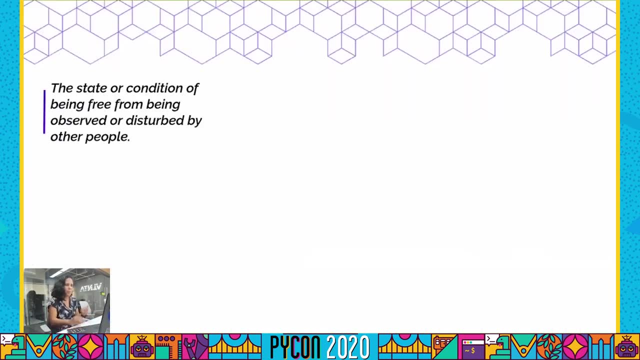 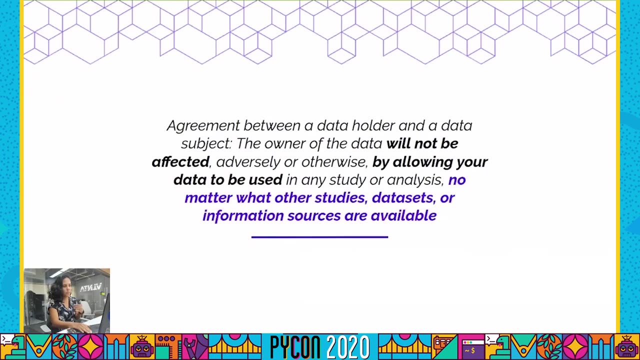 still need private information is like: how can we do, how can we make like consults on a data set private? and there's a lot of people that talk about definitions of privacy and there's a lot of people that say a lot of different things, but one definition that I think. 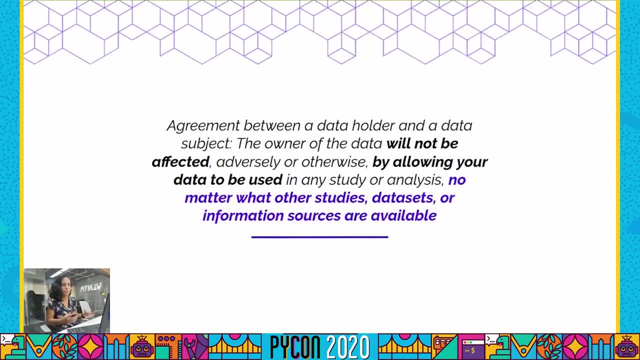 that suits well. our situation here is this one: that privacy is pretty much an agreement between a data holder and a data subject, and the agreement is pretty much that the owner of the data will not be affected by allowing the data to be used. the critical part is, no matter what other studies, data sites or information. 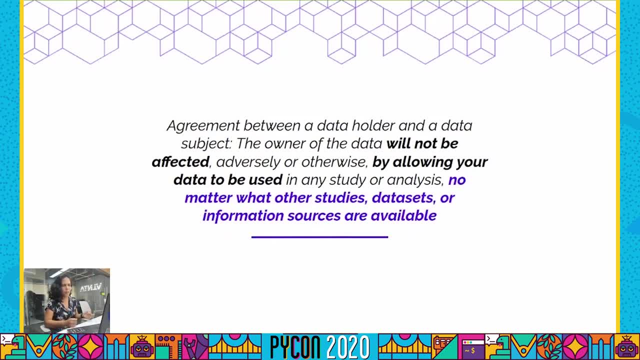 sources are available. so this is kind of critical because before you remember that we were concerned about other information appearing and people being able to do like links between the information and this definition kind of says this is not important because you'll have something that will protect you against the data and it's not important because you don't have. 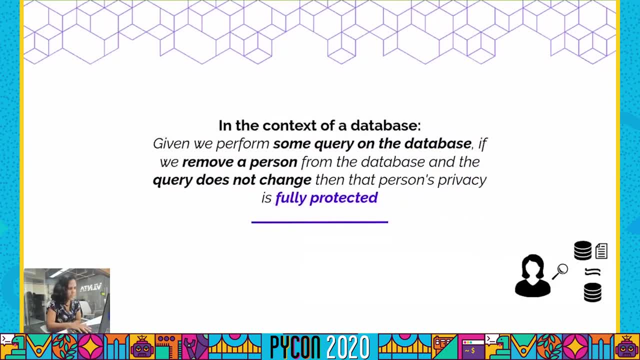 this other information that may appear in the context of a database, what this means. the idea is that you are doing queries over your data set and if you remove one person from a data set, the result of your query will not change. then the privacy of the person is fully protected, so an attacker is not able to know if 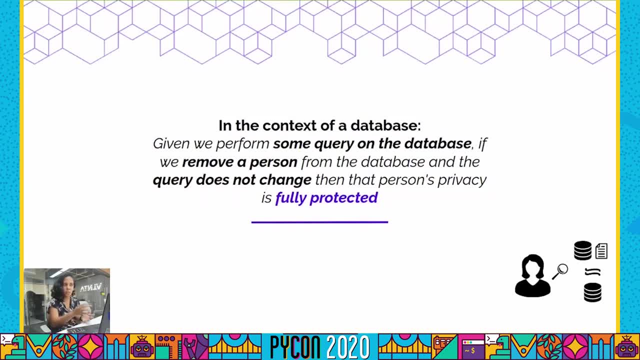 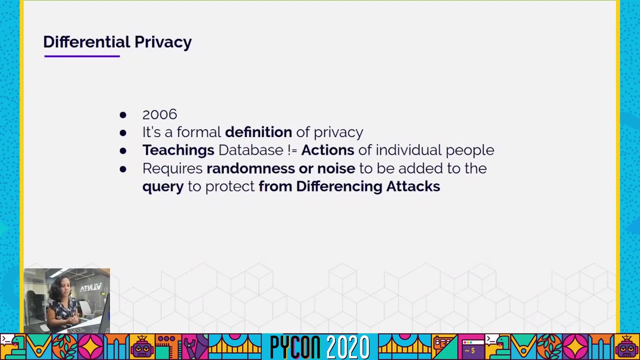 he's doing queries on a data set with your data or with our data. so this gives you, this gives us, a kind of plausible liability of the presence in the database as well. the name of technique, the state. this is called differential privacy is a technique from 2006 and it's a formal. 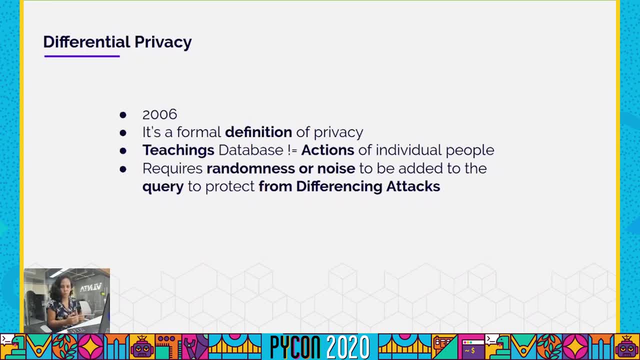 definition of privacy and I will show you the equation. and the idea is that you can learn about the teachings and the underlying information on the database without learning about the actions of individual people in a database. and it does that by adding some kind of noise in the query to protect from. 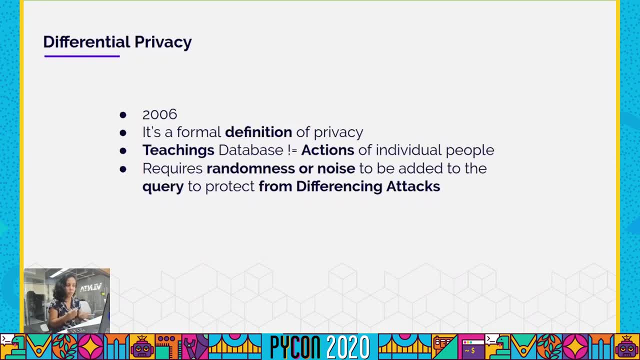 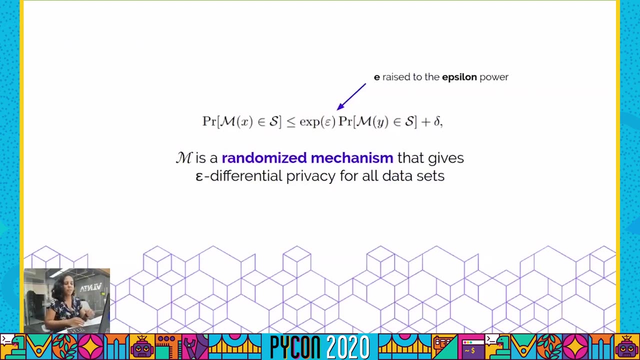 differentiating attacks. so adding the noise is kind of randomness or like a random mechanism is kind of the critical part here. I'm gonna show you the formula now. bear with me with this. here the idea is that we have a term on the left and this term just means that we have one data set and we have a protocol that 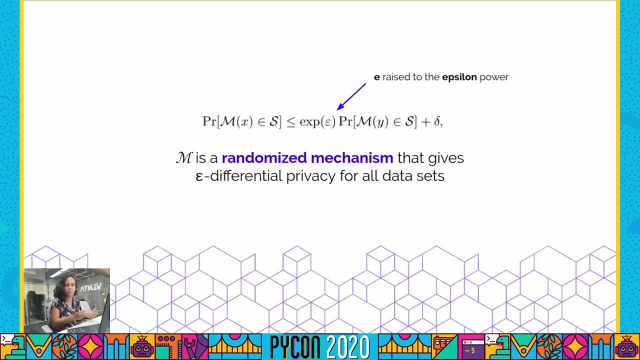 does queries in a data set and these queries just have private results. and the term on the right is that I also have a data set, but it's only different by one, and I have another protocol that does queries that gives me privacy. the idea is that these two terms. they differ by eraseDepth of power. 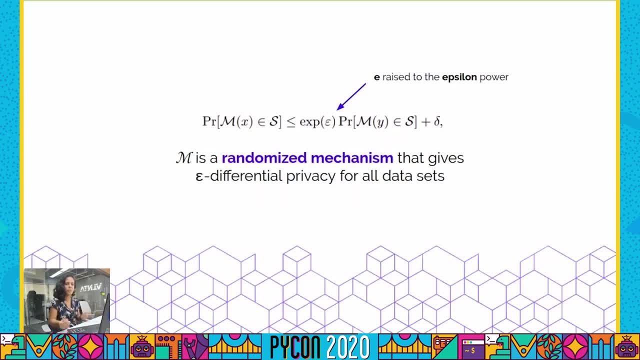 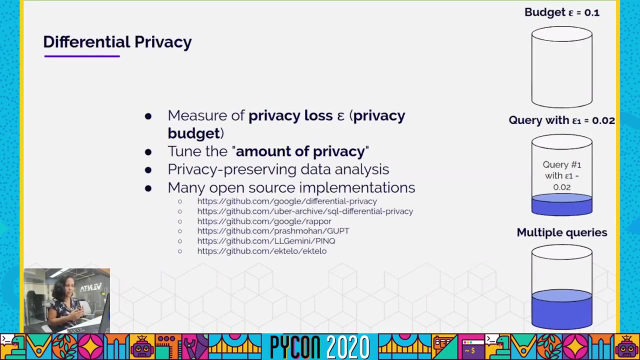 which is a very small number. so when you're doing queries of both data sets they are like pretty much the same, and this epsilon variable is fairly critical here because it allows us to like tune the amount of privacy that we want for a project. so we have a way to measure the privacy loss that we have when doing queries and we 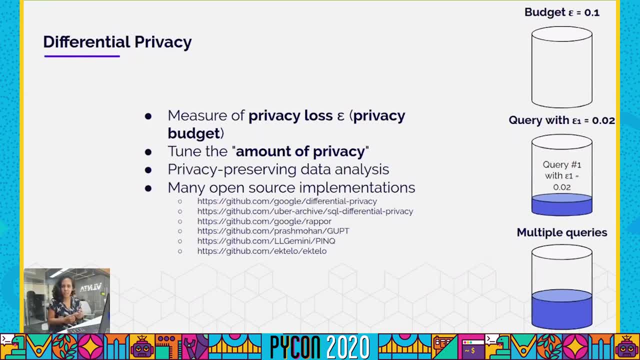 have a way to define a privacy budget which is like critical for like many projects, so I may define that above a set or certain level, I'm leaking too much privacy and will not be safe for me to allow people to do consults on this database. and another interesting thing about this technique is that we have, like many, open source. 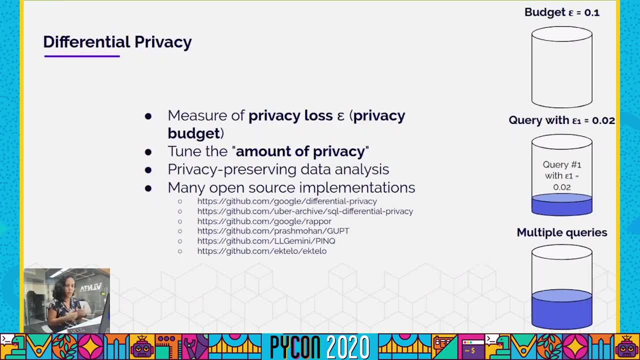 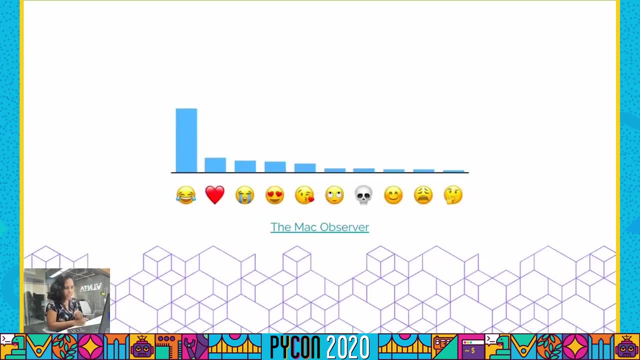 implementations and they are like pretty much amazing. I will like recommend you to check that later. a nice application of this technique is most use emoji. it was developed by Apple and apparently we have smiley and crying face as the most used emoji and in second place is heart. 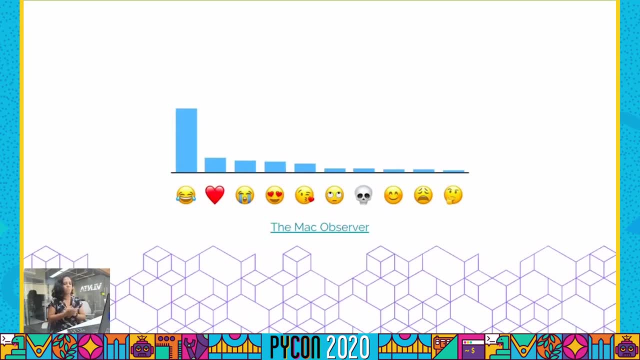 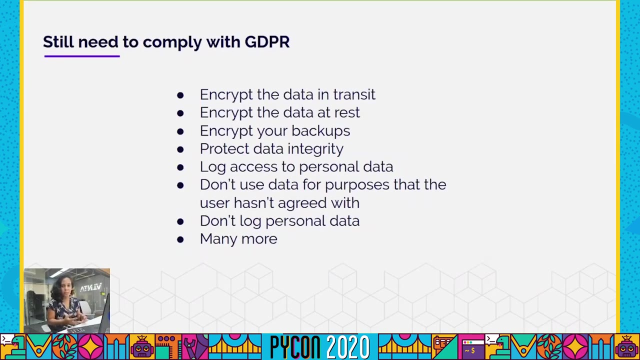 emoji and these techniques. they will be like your best friends when you have like regular applications and they will help you assure privacy to users. but I would like to remind you that if you are using data from like European citizens or you're bound by a few regulations, there's still a few more things that you need to. 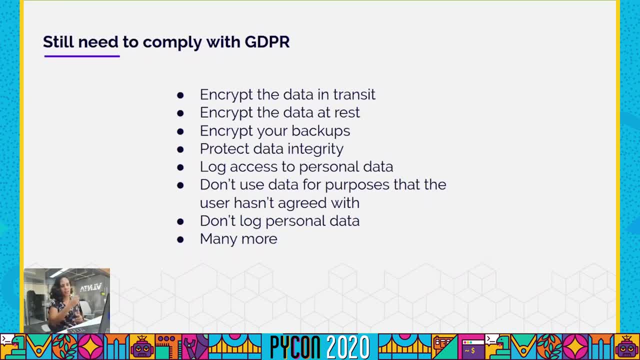 comply with. so you need to like encrypt data to all of the safeguards that the regulation like ask you to do so still need to give it a look on the regulation, don't? the second will help you, but you're still gonna need to like go one step further in order to like comply with the regulation. 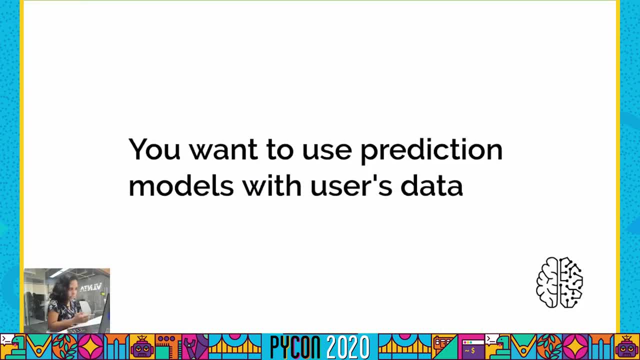 okay, another situation that I would like to talk about is, like phenomena build prediction models. we talked a little bit about like regular business models, but we have like new business models that like rely on, like prediction models and artificial intelligence and machine learning. how can you do that while like 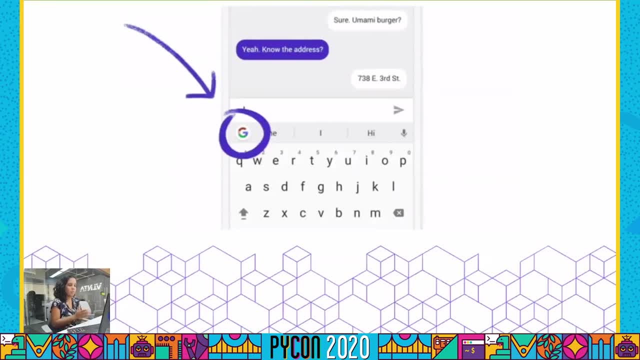 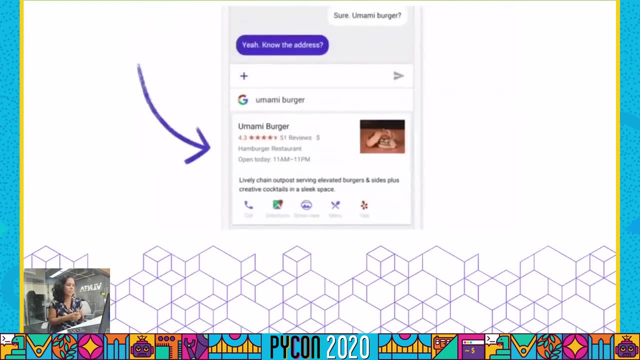 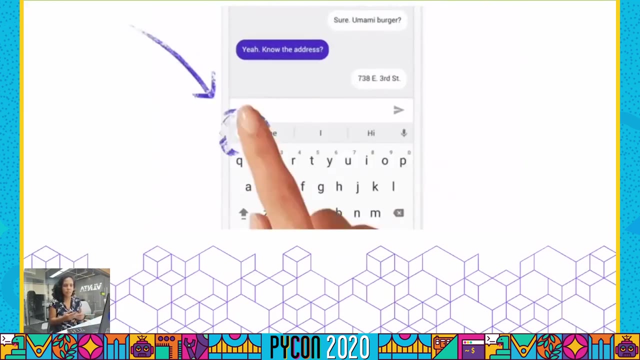 ensuring users privacy. one example of applications- just so we like getting to the moon- is when you type something on your keyboard and it tries to predict where you're typing. so this is an example of a prediction application that is like mobile phones and that we use pretty much. 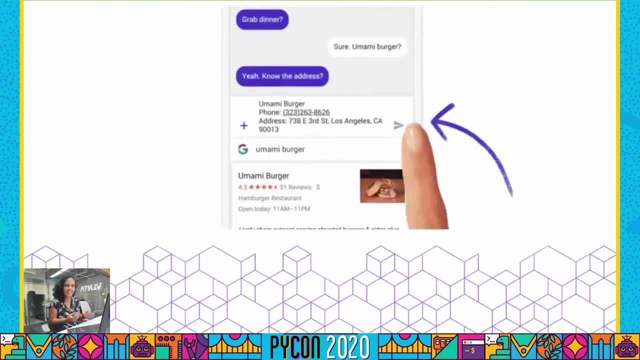 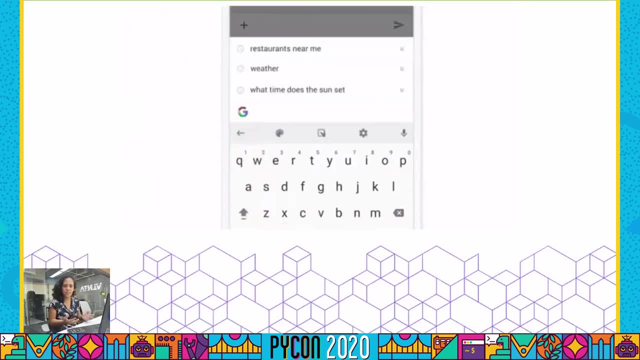 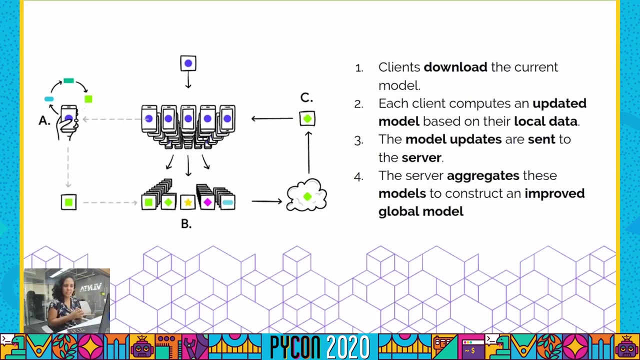 every day and mobile phones they kind of get, they kinda have all our life in it. so how can we show privacy in this context? so the idea is that if you're a big company, you just sell and send, like put machine learning in people's phones. what you do is that you build one model and you'll then share this model with many clients. 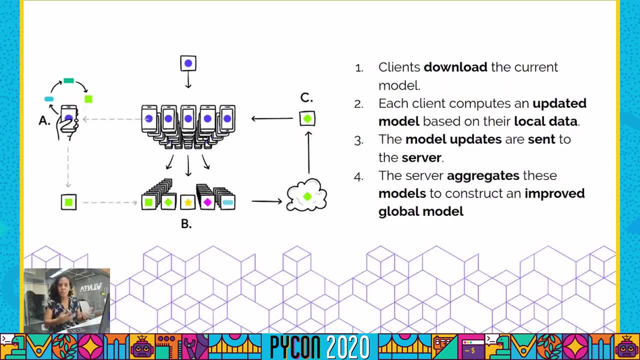 unlike us and your clients, they will use this model and they will interact with this model and they will change and customize this model locally and at some point they will have like a new model. and when you have like a good amount of good models from different people, you send these models to the server and the server will then 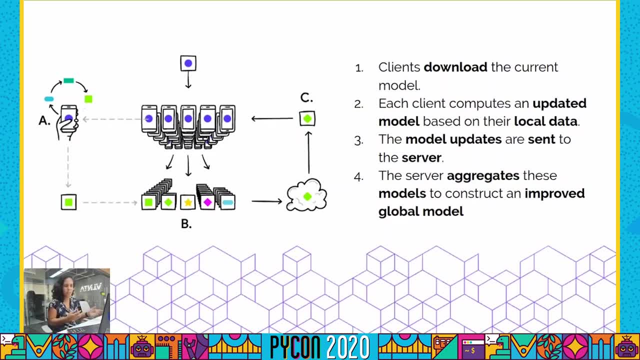 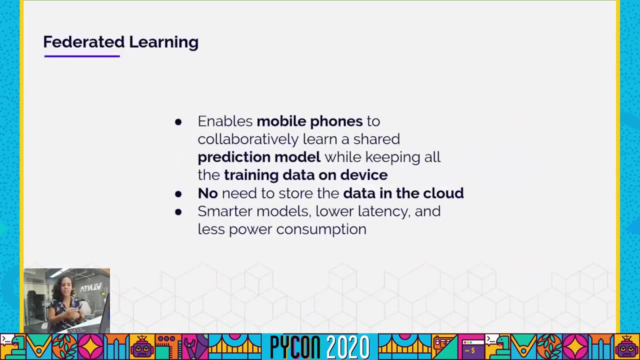 aggregate these models without ever seeing the customers information, and generate a new model and send back to the users. This technique is called federated learning and the idea is that mobile phones they can like collaboratively build prediction models while keeping the training data on device, so you never, ever, ever send. 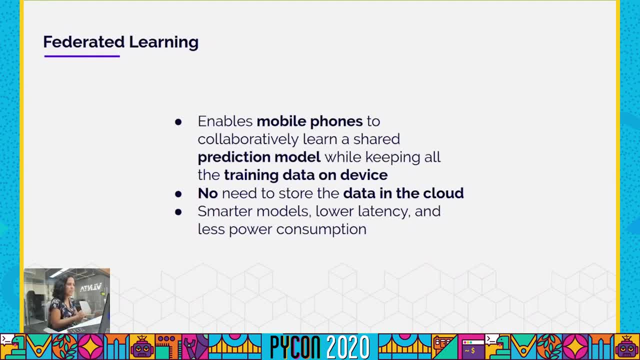 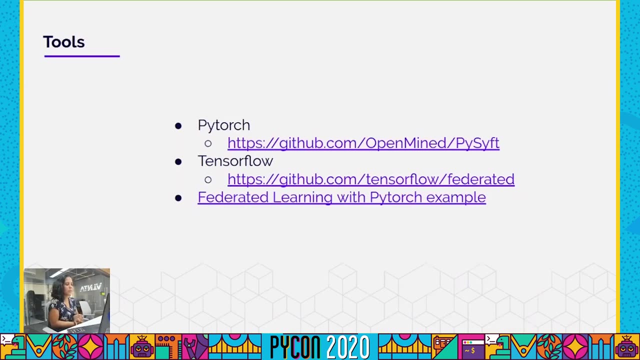 customers data to the cloud, and this was a technique developed by Google, if I'm not mistaken, and they say a lot of things. they say that it gives you smarter models, lower latency and a lot of good things on that. There's a few tools that you can do this on. 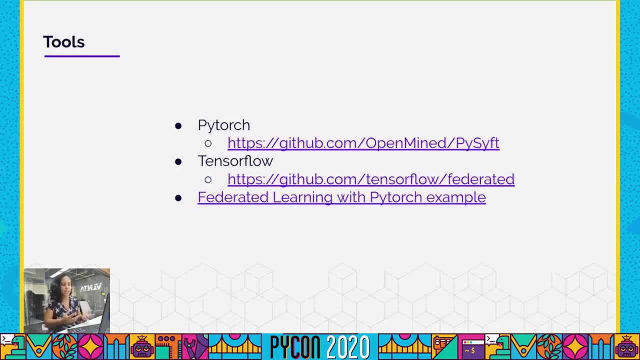 Python and they're all amazing tools. I have tested a few of them and I have left you a link with some implementation here that you can check. Just a simple example: how you can use federated learning and send like a call to clients and they will execute and then send the results back to you. 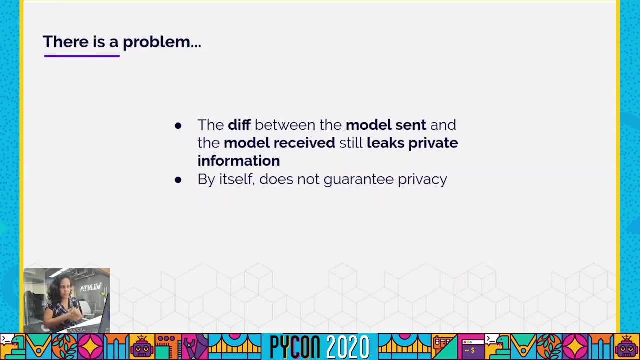 Okay. so this is a problem and if you were like some person here, you may have seen the problem. it is that you can still infer private information between the models. the server knows the model it sent to and it knows the model you received. you still can like infer some type of private behavior from the user. 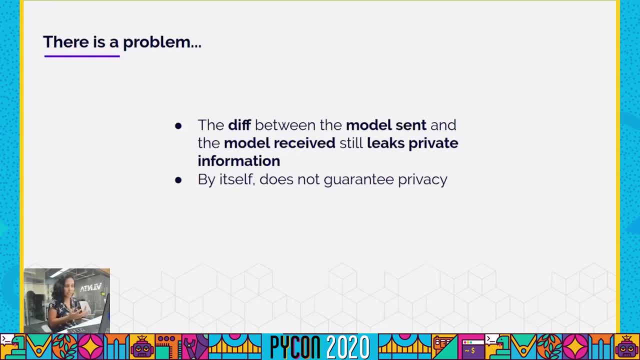 and get some type of private information. So this technique by itself does not assure your private behavior from the user and gets some type of private information. so this technique by itself does not assure your private, But it's a good way for you to start and it should be used with other techniques in order to assure privacy. 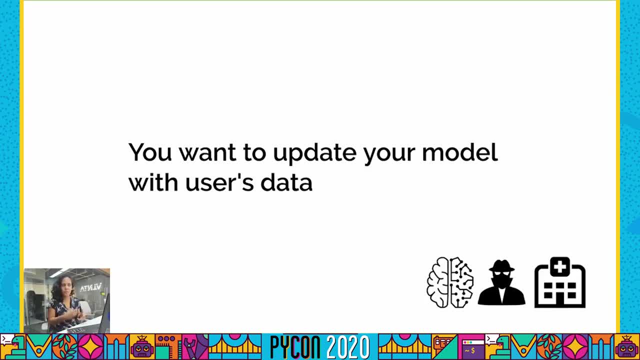 But you still want to update your model with user data and user data might be like many users and It still is a critical part for your business model to like having your data updated with data of a lot of people And this is critical, like for hospitals, because they can't just legally. 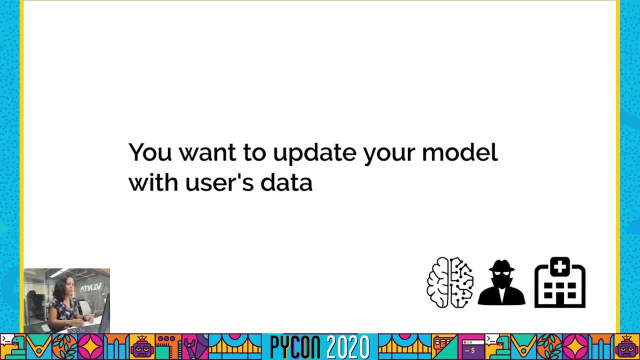 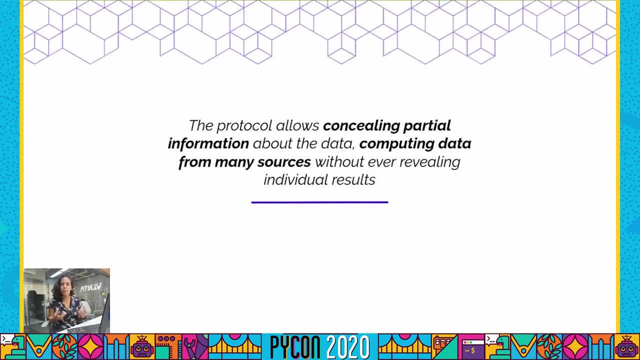 Hand over the information to all the hospitals, or the same thing for intelligence agents, But how still they can like cooperate without like sharing private information? This is a critical point. The way that we can do this is that we create a protocol. They allow users to conceal private information. 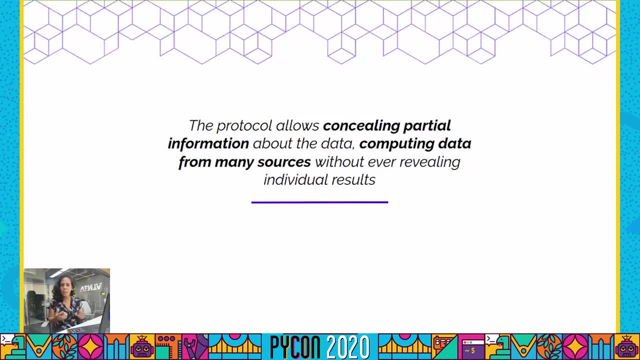 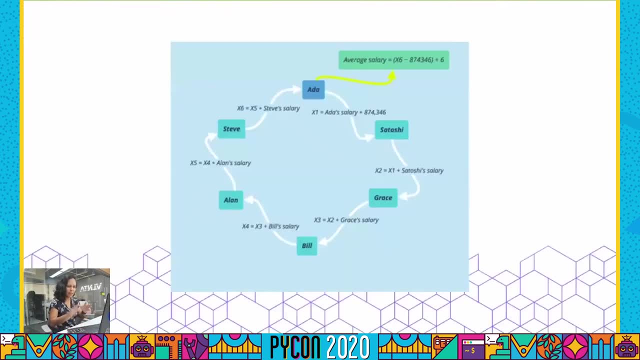 Usually in a encrypted matter, and you can make computations over many sources of data without revealing the individual results, and I have an example of how this would work. Let's assume that I have a system with six people here and I want to know the average salary of this person. 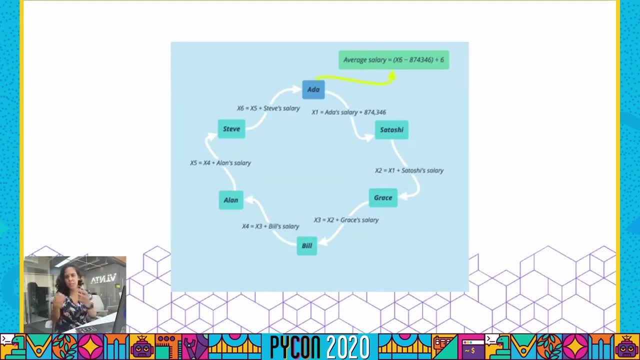 So I don't have a trusted third party to just give all the information. Then this third party will return to me the result and don't have them. The way I would do that is I'll have the first person to just get his own salary and just. 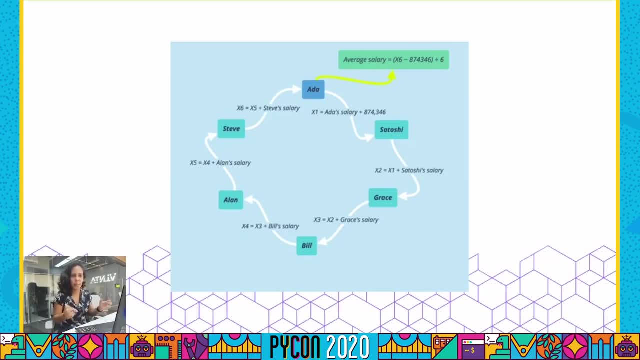 Add a big number- in this case I'm kind of cryptographic- And the the salary in there on pass to the second person. this person would then add his own salary and they will pass to the third person and everyone will add up the salary to the initial value, to the value that the previous person passed it and 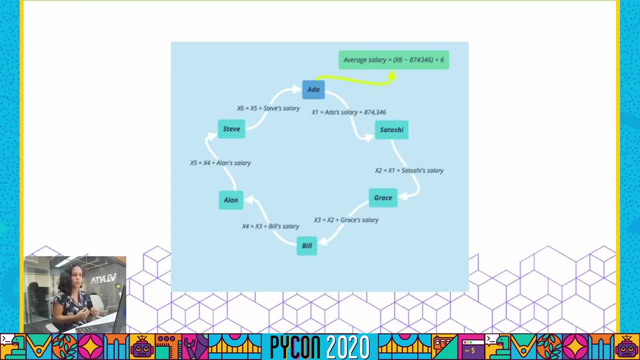 The final number will then come back to the first person and this person will then decrypt, Like the number by removing the big number that she added at the beginning, and then perform the operation. So in this case it's an average- and then we'll say the result to everyone and 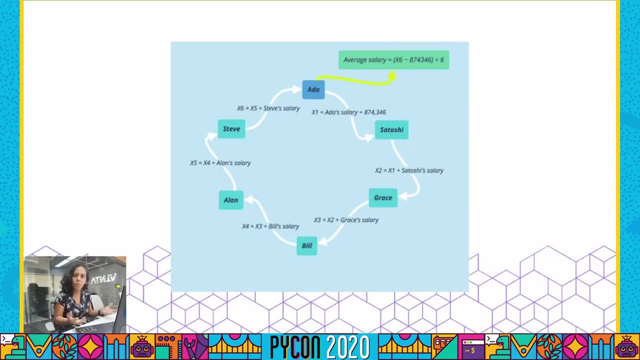 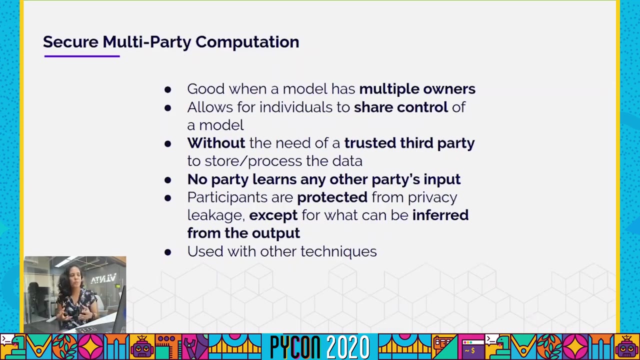 The advantage of this technique is that everyone will know the average, but no one will be able to tell which. What was the salary of the previous person or the next person, or anything like that. So the name of this technique is called Secure multi-party computation, and it's amazing when you have multiple owners to have, when you have multiple people. 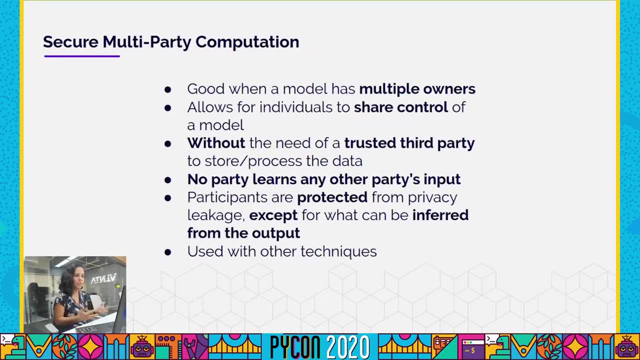 Building models together and allows for individuals to share the control of the model without the need of a trusted third party. No party learns any other party's inputs, and that's critical, And the only thing that the persons, the people involved, they can like infer is what can be inferred from the output. 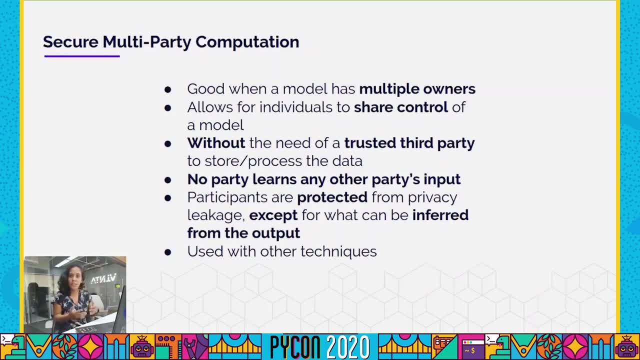 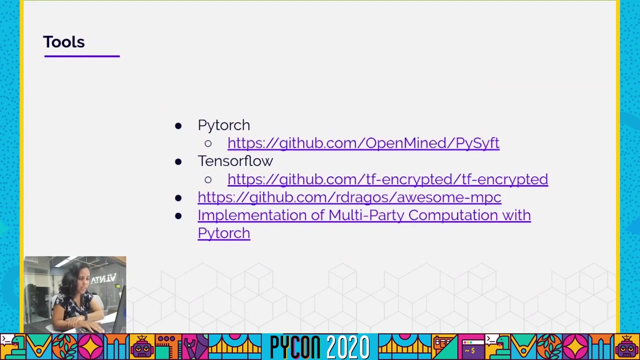 And it's usually used with other techniques. This technique can be used jointly with federated learning to assure privacy in the processing of. It's like updated with machine learning models of mobile phones, and There is also like amazing tools for you to do that. I have laughter on some examples here and there is as one limitation here. then you can check this link. 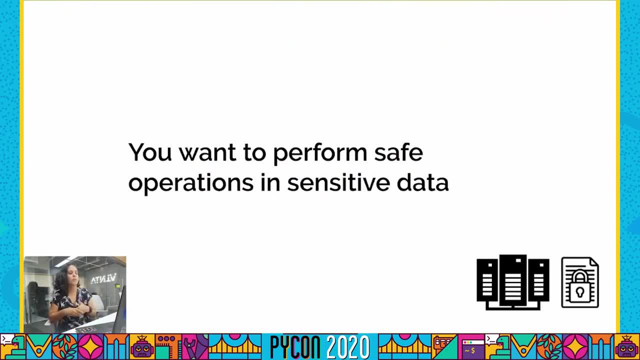 Sorry, The last things in a situation that I would like to talk about is that sometimes You can, you don't have multiple owners. you're the owner of anplate. many times you can't make two cases at once with single owners can keep together on Inster- ens relacionadas por determinadas reuniones e contadas porRETAM caraçõesmos a cada vezmos. Más cosas como situações são Today's point- this is something that I'd like to talk about- is that sometimes you can't, you don't have to call on this. you weren't being ordered on your account. 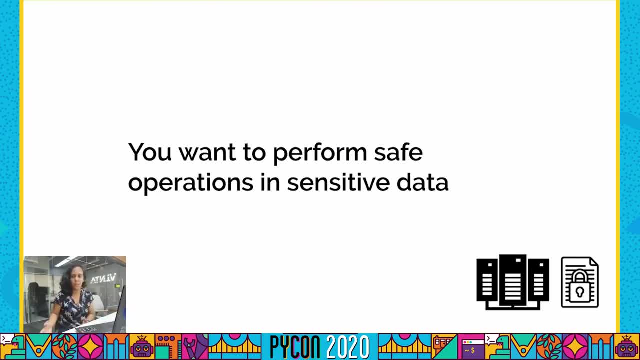 the data, but you can't download your data and process on your machine, or you can't process in the cloud because it's not safe or because you just signed a contract and you can't have other persons processing your data. How can you do that in a way that you still follow the law? 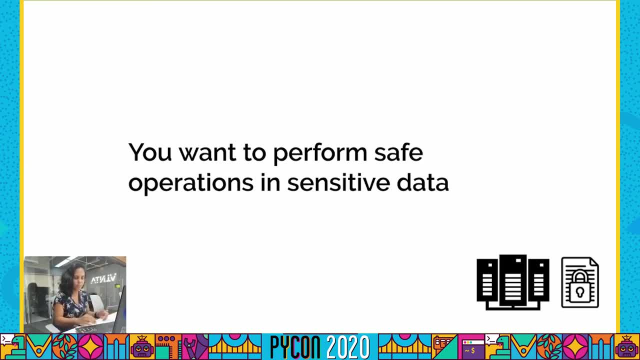 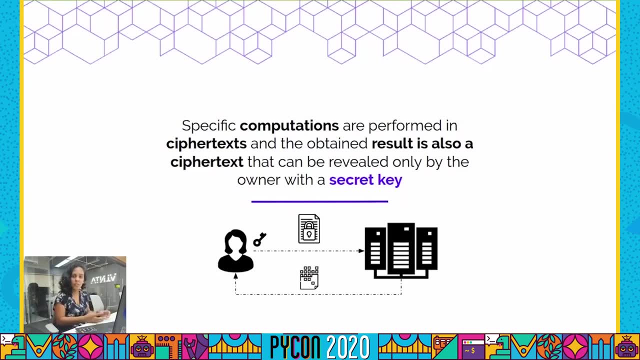 still follow the regulation but still get the results that you need. There is a technique that it allows to perform some types of computations on ciphertext, so encrypted data, and you can obtain results in encrypted format, and these results can only be decrypted with the owner of the secret. 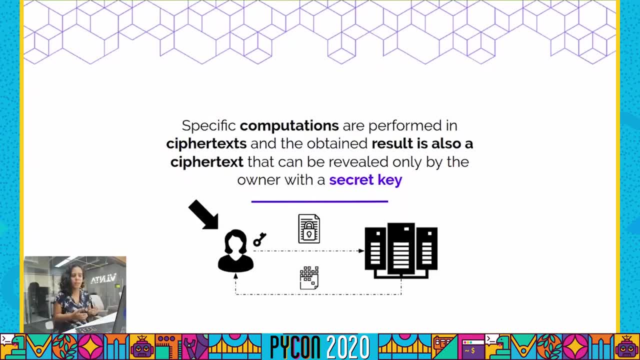 field. So it's good for the user because it just gives me the security that if I encrypt the file and I give to a third party and this third party will perform some kind of processing and this third party will not be able to access the data. 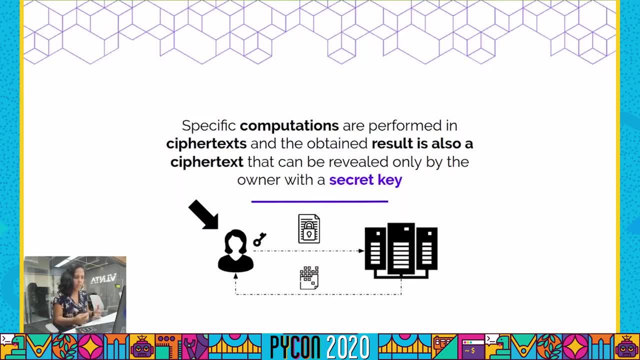 The information that I'm sending him, because it's encrypted, and the results that the third party sends me will not be like. the third party will not understand the results because they will also be encrypted and only me, with the secret, will be able to decrypt it. This model is also good for the 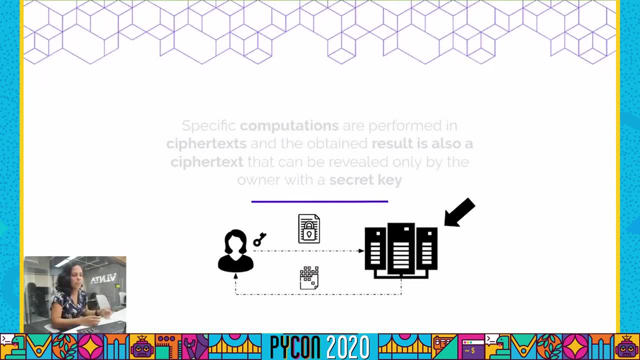 third party. because let's assume that you have, like, a prediction model that is like amazing, top-notch and like very innovative, and you want to protect your data, so, So you would encrypt your model and then other people would be able to train and use the results of your model. 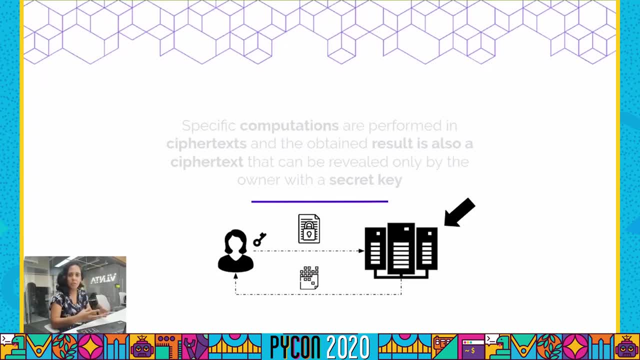 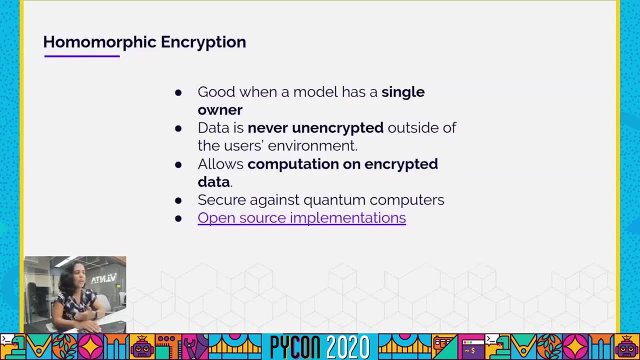 without ever seeing the inner behaviors of the model or stealing the secret sauce of the model. The name of this technique is called homomorphic encryption, and it's good when a model has a single owner, because the idea is that data is never only encrypted outside the user's environment. 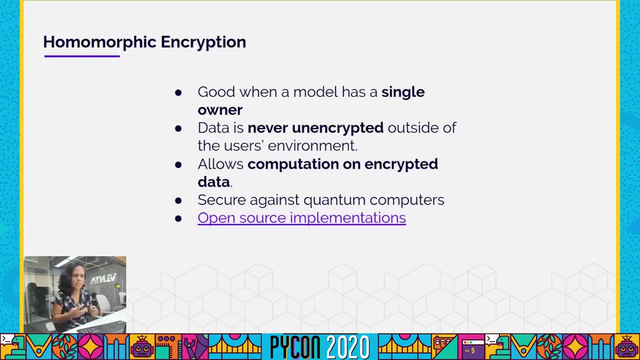 It allows computation and encryption data, and this is like the critical part, because you can get encrypted results that only you, the owner of the secret key, is able to decrypt. This technique is also- people say right, I'm not, I didn't verify, but it's secure against quantum computers. 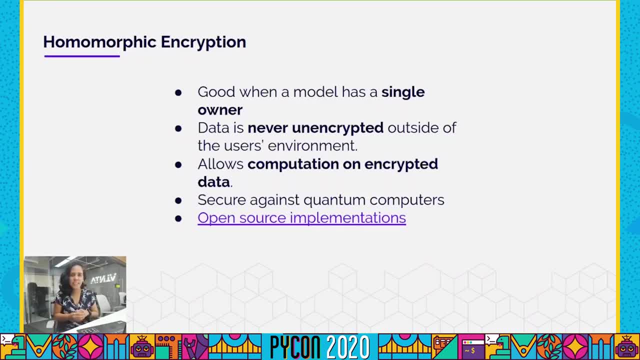 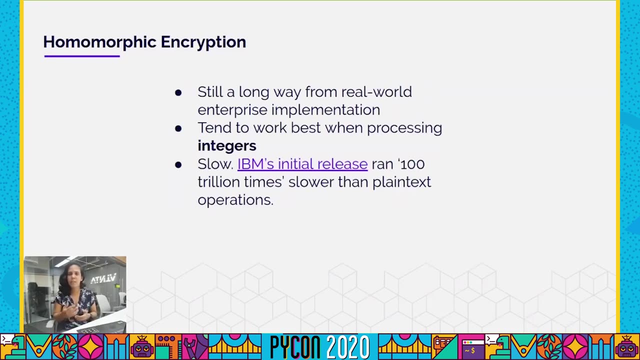 and we have a few open source implementations, and I think that this will be like the technique that will like give you the best results: Private processing data in the future. Can I say that in the future, Because we're still a long way from like production use. 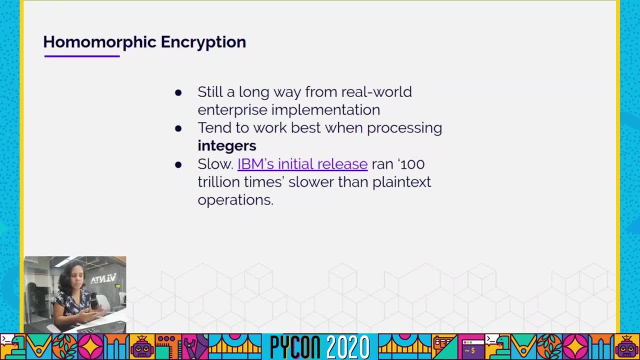 Pretty much because data, this type of processing, works best with interviews and initially it's still like pretty slow. so there's a few scaling issues. If you do with a small amount of data, it might be okay, but if you have like a big amount of data, 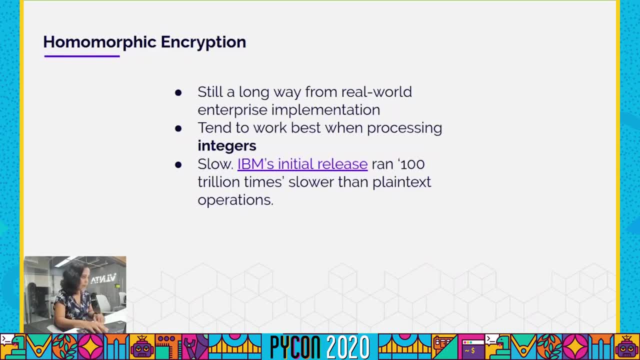 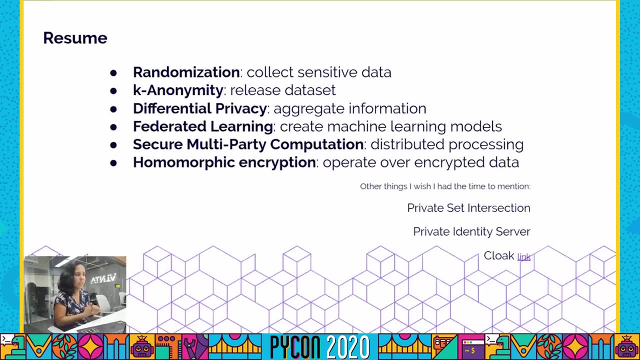 it may be very difficult. It's very difficult for you to use this technique. So a resume of what we have discussed today. We have talked about randomization to collect sensitive information. Canon immediately release dataset. but be careful with this Differential privacy if you want to do aggregations and consults. 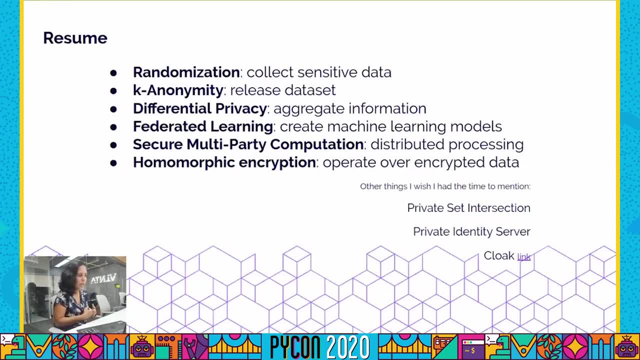 Pretty much to privacy, data analysis, Federated learning and secure moving-party computation if you want to do like create prediction models and machine learning models using data from science. And on mapping, encryption, that allows you to make operations over encrypted data And this technique may be like the way that we solve privacy issues in the future, but not yet.